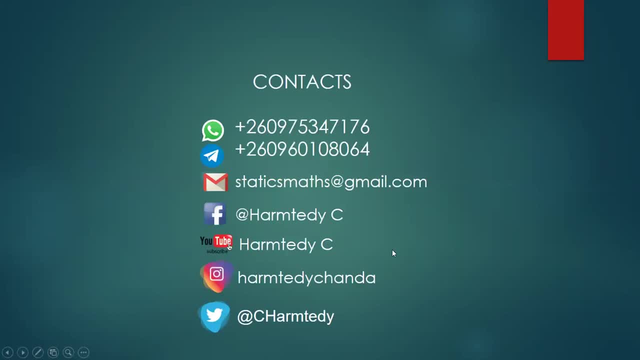 these are my contacts here on the screen, so you can just text me either on whatsapp, telegram, you can email, you can text me on whatsapp, rather on facebook. this is my youtube channel, and then there's also, if you want to find me on instagram. this is my username, is hamte chanda. 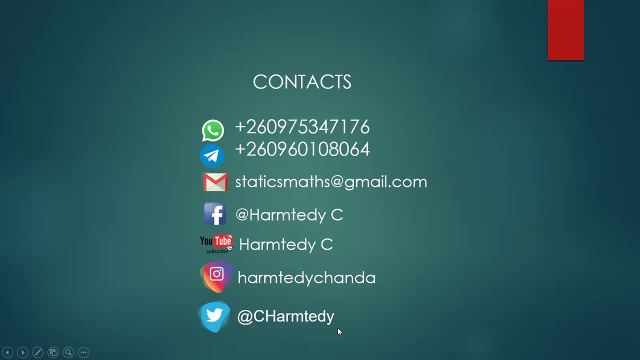 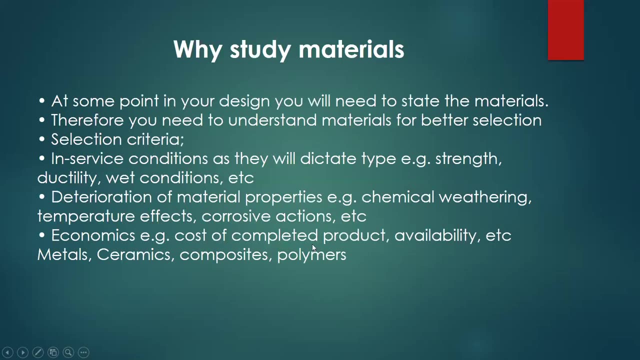 on twitter is just c hamted. yeah, so that's, that's it all right. so let's quickly begin to learn. so one thing you have to know, apart from knowing the topics that you're going to cover in materials, one: you also need to know the reason why you need to learn this course. so 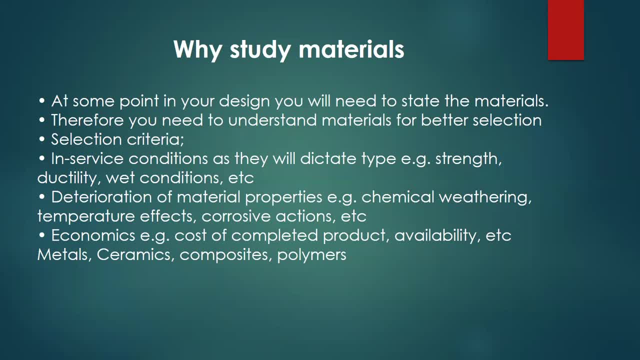 from the word itself, materials. this implies that we're going to discuss or we're going to learn different, different types of materials that are used in engineering. yeah, so, be it electricity, I mean, be it electric engineering, mechanical or any type of engineering, civil engineering, you need to know the. 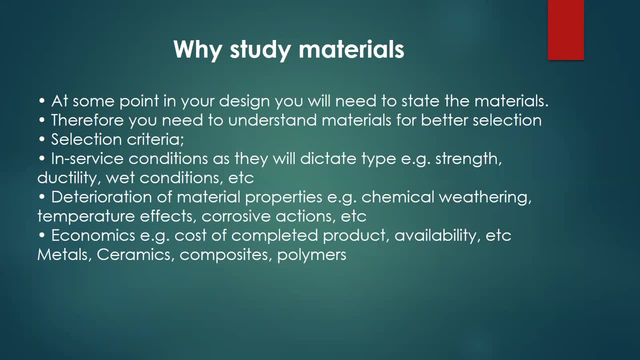 type of materials that you are going to use, and one of the reason why you need to know the type of materials is this first point, yeah, so, which is, when you're designing anything, when you've been taught to design anything in engineering, you need to know the right material that you are going to. 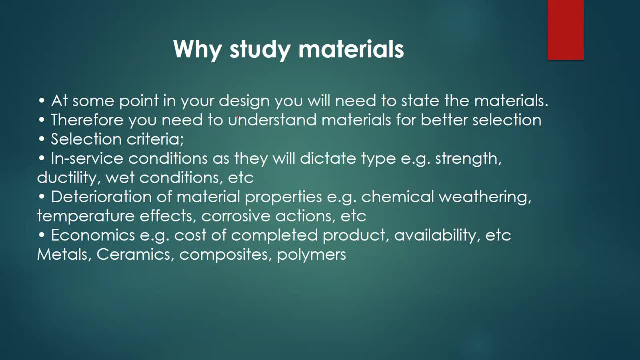 use to, to assist, to design that, rather to to make that material. yeah, so in designing, when writing down all the requirements that are needed for a particular machine or a particular component to to be manufactured, you need to know the right materials and their properties. yeah, because you. 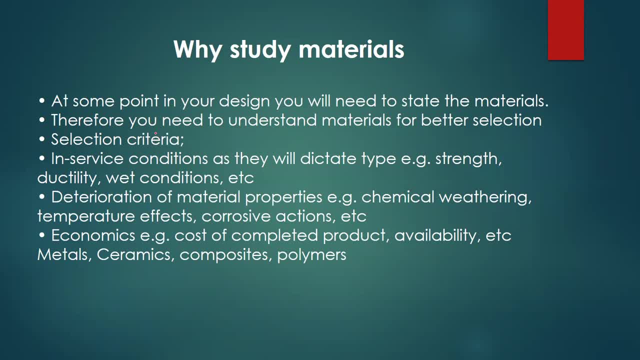 you can't know something or you can't tell, to say this is the right uh thing to do. rather, this is the right uh thing to use if you don't know its properties. hence, this course helps, helps us to understand the physical, electrical and chemical properties of different materials. so we're going. 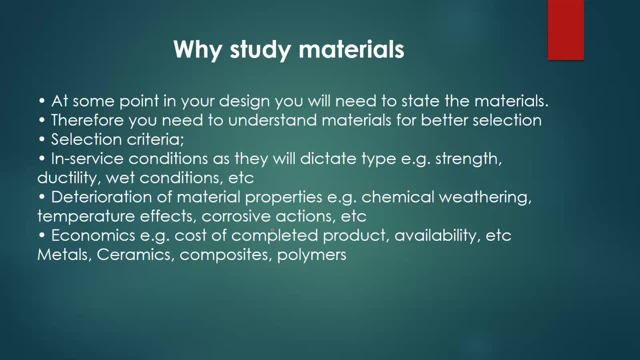 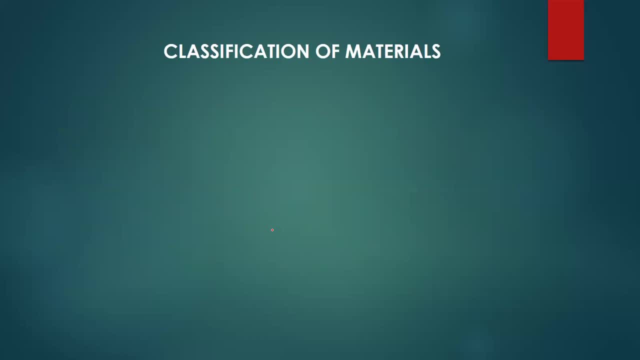 to learn that as we proceed. all right, so let's quickly look at the classification of materials. so basically, in this course we're going to discuss three types of materials, from the start up to the end. then, apart from that, we'll also look at the economical, the economical way or the economical approach to these materials. what do i mean by that? 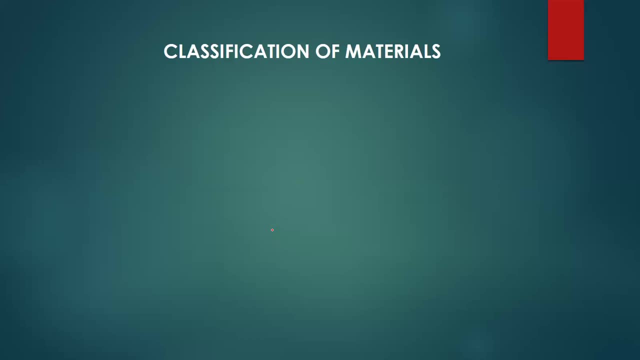 i mean the cost of these materials at the market and then, apart from that, to also look at the availability of the materials at the market. that is, i think it's going to be our last that we're going to cover, And I believe we're going to do that before we open. 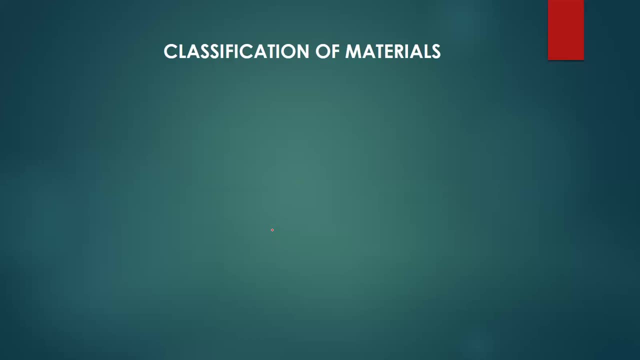 I want us to at least move. If anything, we should finish the syllabuses before we open. All right, so classification of materials. So materials are classified in three classes. So the first class that we have are metals. So we have materials which we all know. 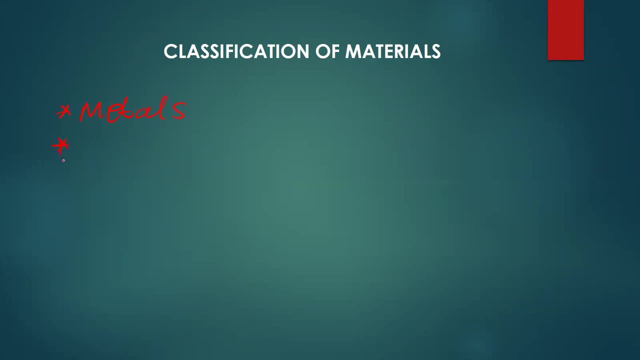 which are called metals. Then, apart from that, we also have what are known as ceramics, So ceramics are also materials that we're going to discuss. Then, apart from that, we also have what are known as polymers. So I believe you guys learned polymers in chemistry. 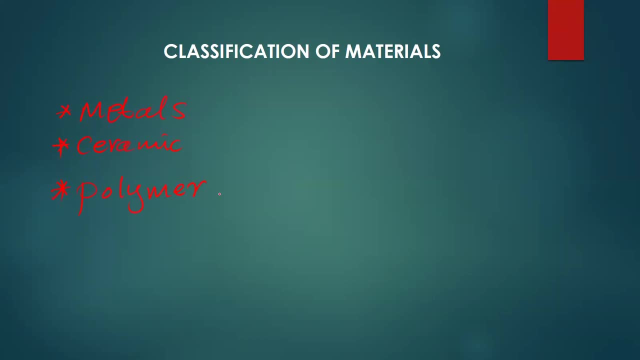 So, the same polymers that you learned, the polyvinyl chloride and other polymers that you know, they are the ones that we're going to discuss in details, Their properties and their applications, where they are used, and everything. So this lecture slide is just going to introduce us. 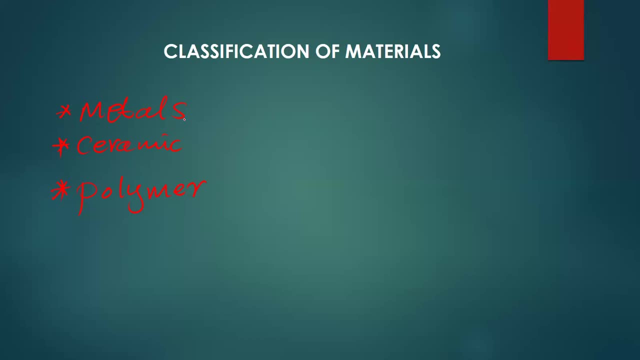 to all these three And then, as we proceed, we're going to be looking at the chemical, the chemical properties of metals, the physical properties, And then we'll also look at other properties of metals that will make them good for particular uses. 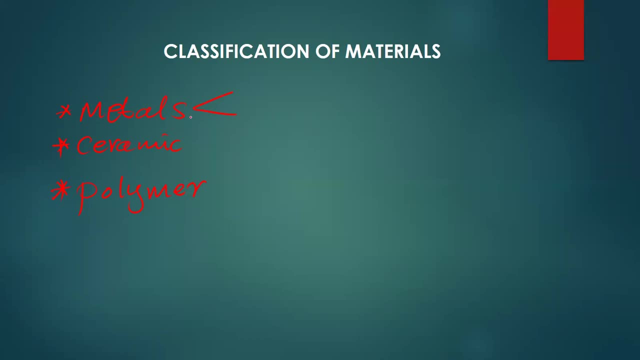 So, and then, apart from that, we'll also look at some calculations, Like finding the stress, the strain of these materials. So we have a lot of things we are going to be looking at. the factor of safety: Yeah, so how do you know that what I've created is safe? 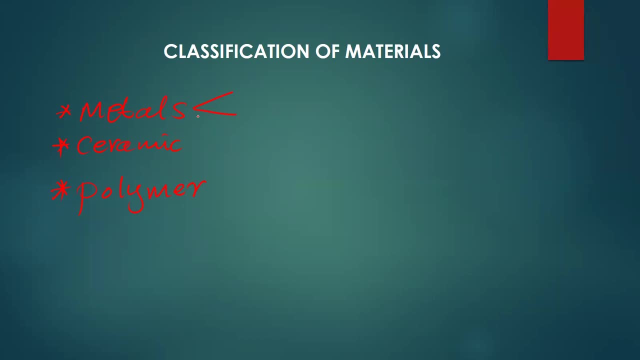 How do you know that what I've manufactured is safe? You look at all those properties. Yeah, so we have a lot of properties that we're going to discuss, which will help us to move, or rather to come up with a good solution. 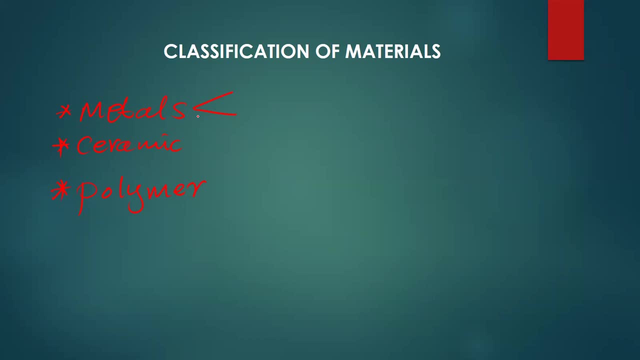 with a good machine or a good- I don't know anything- that you are making, anything that you're manufacturing. Yeah, so this is basically the introduction. Material science is the introduction to manufacturing and technology. For those that are doing mechanical engineering, 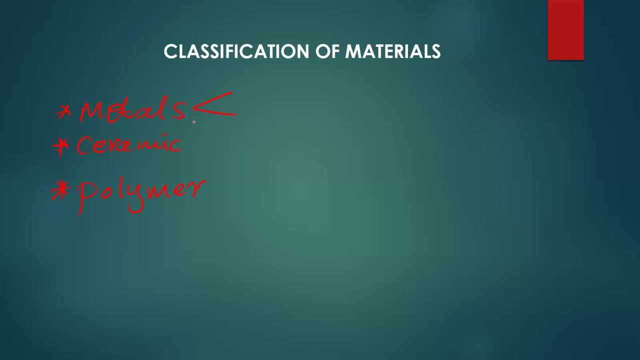 are going to do it in your fourth year. Yeah, actually you do man tech in, I think, third year, semester two, and fourth year, semester one. All right, so I'm going to look at metals and then we'll also look at ceramics. 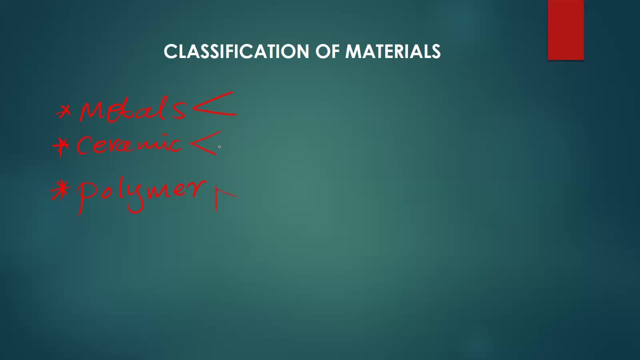 Then, apart from that, we'll also look at the polymers. So let's look at them one by one. So today we're just doing an introduction to this, and then next time we'll go in details. And then, apart from this, we also have what are known as the 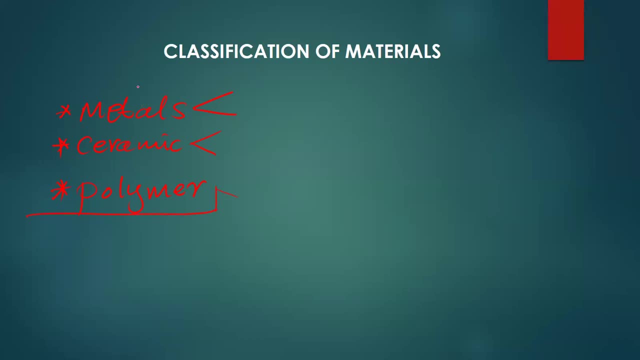 okay, we'll look at them, Because when we look at these metals, ceramics and polymers, there's a way we call so we can combine them to form other materials. Yeah, we know to say when you combine two or more metals. 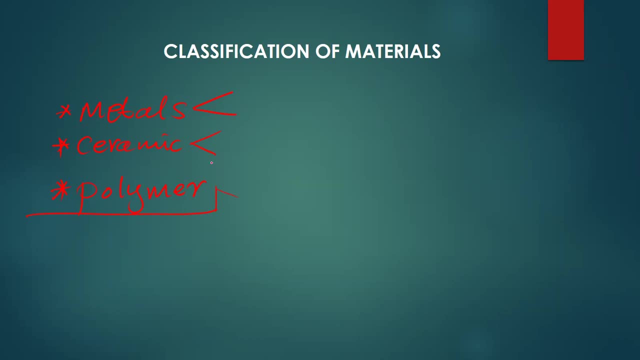 you form what are called alloys, Then we also have what are known as advanced materials. So advanced materials, these are the materials that are used to make things like the ICs, those components that are found in computers, and the micro and nano components that are found. 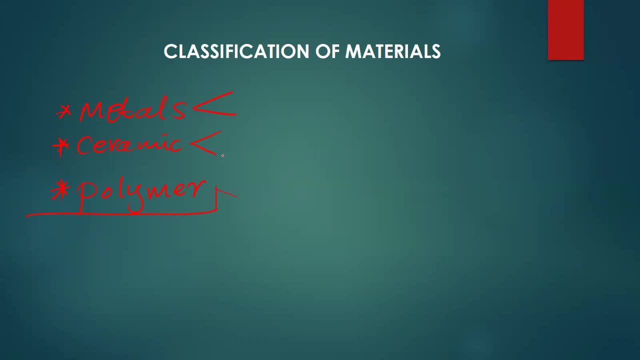 in electronic components. And then we also have a lot of things. Yeah, So let's quickly get into discussing the details of these things. Okay So, let's quickly move on. So we have these are just okay so. classification of materials. 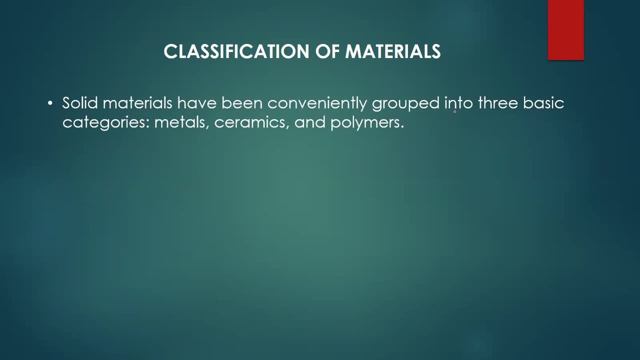 So these materials have been conveniently grouped into three basic categories, that are metals, ceramics and polymers. So I've talked about this. and then this scheme is based primarily on chemical makeup and atomic structure, and the most materials fall into one distinct grouping or another. 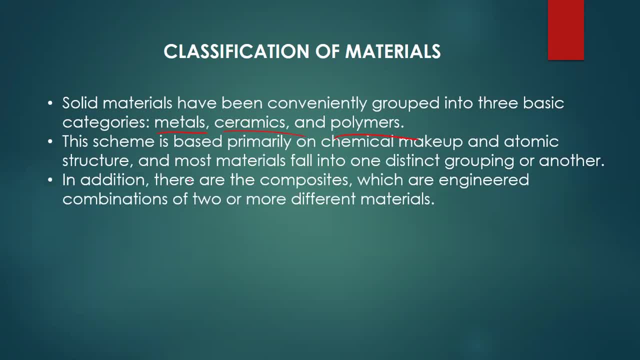 Okay. So I'm just reading through the notes, or else of these I've explained. I've explained most of the things, Okay? So, in addition, there are composites, which are engineered combinations of two or more different materials. So remember what I told you. I said there's a way you can combine. 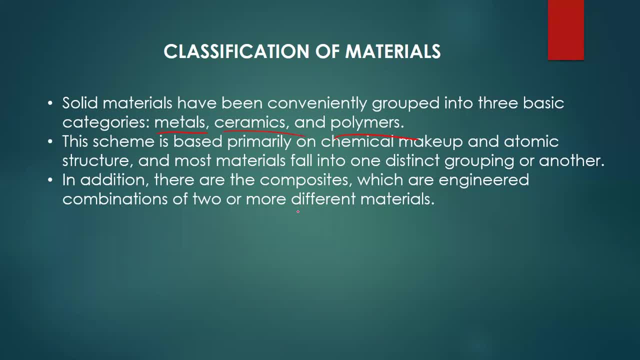 there's a way you can combine metals and polymers. there's a way you can combine ceramics and polymers. So, whatever that you form after combining any of those two or three, I mean two or more basic, I mean classes of materials. 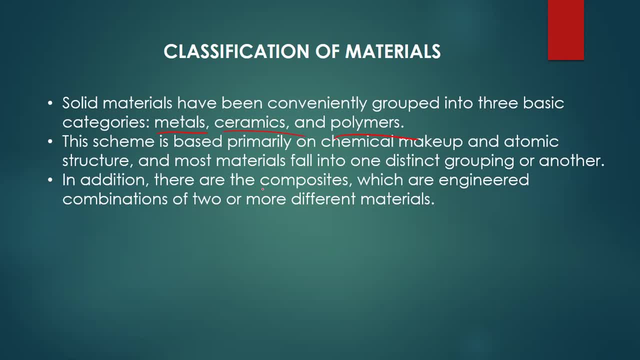 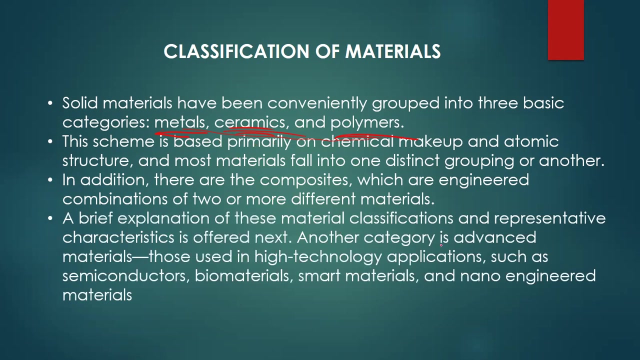 When you combine two or more, you form what is known as a composite. Yeah, So composites are formed from combining either this or that or the three or this or that. I mean the result is known as a composite. Okay, So we also have what are known as. we also have what are known as advanced materials. 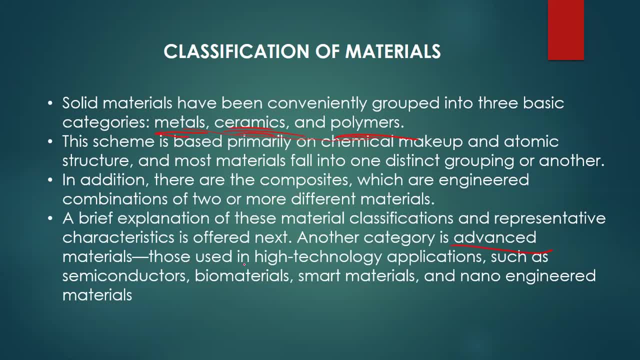 Yeah, So advanced materials, I'm sorry, Yeah, Okay, So we have a composite. these are used in high technological appliances. So I mean applications, So I talked about this- high technological applications, like making the ICs and making those very small components. 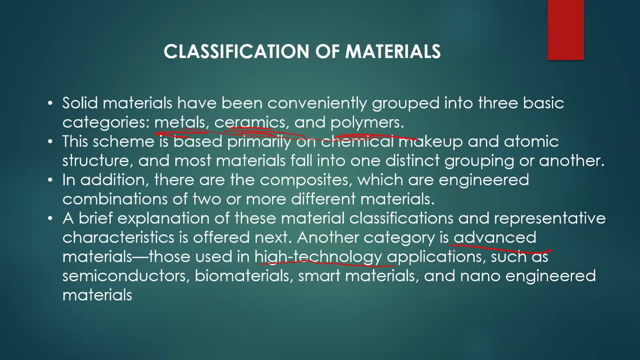 of electronic devices. They are made out of what are known as advanced materials, And then these advanced materials are known as semiconductors. I mean examples are semiconductors. We have the biomaterials, And then we have the smart materials. 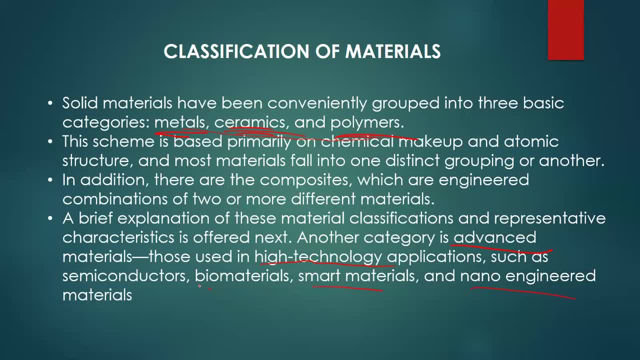 and then nano-engineered materials. So when you talk about biomaterials, these are simply what can I call them? They are just replacements of a human body, or not only a human body, but of, I think, any living thing. 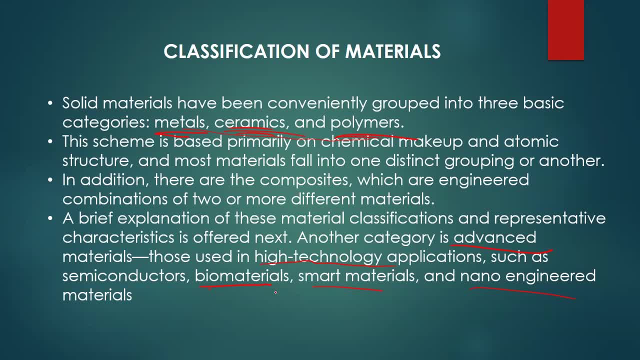 Yeah, they can. I'm sure you guys have seen something like: maybe they are trying to make an artificial organ of a person. Yeah, so these these organs, yeah, these organs, those artificial organs which they make. they are made out of these high technological appliances. 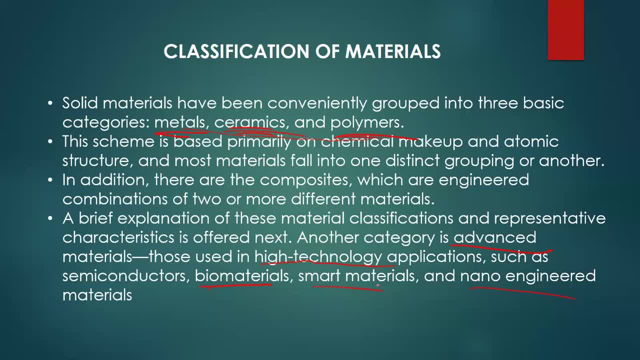 which we are calling advanced materials. Then we also have smart materials. These are, we can talk about smart watches, TVs and everything, yeah, And then the nano-engineered materials. these are the ICs which I talked about, The ICs and other things. yeah. 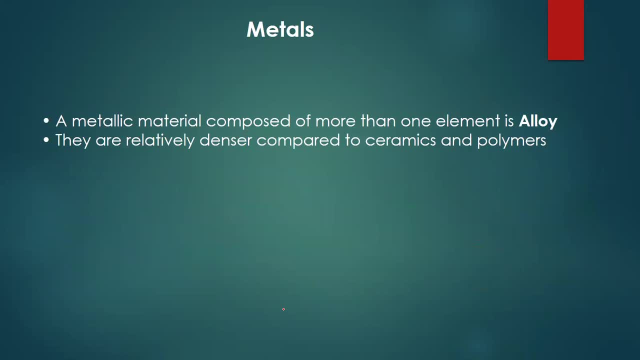 So this is basically what they do. So let's look at them one by one. So we have the metals. So a metallic material composed of one or more element is called an alloy. Like I said, if you have a metal that is made up of one, 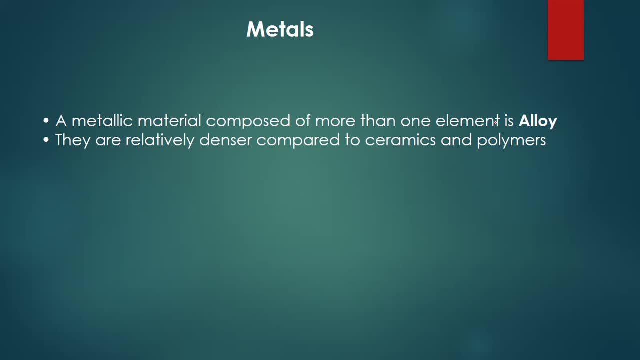 or more, I mean one or more elements. that metal is known as an alloy. yeah, So they are relatively denser compared to ceramics and polymers. So metals are basically denser than ceramics and polymers. Then the other thing we need to know: 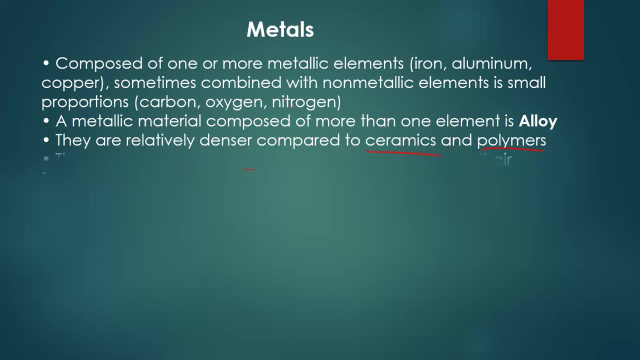 okay, this one has come at the wrong time. Okay, let's proceed. Yeah, so these are some of the properties of metals. Yeah, so metals are made of. I mean, metals are stiff. We learned this, I'm sure, in chemistry. 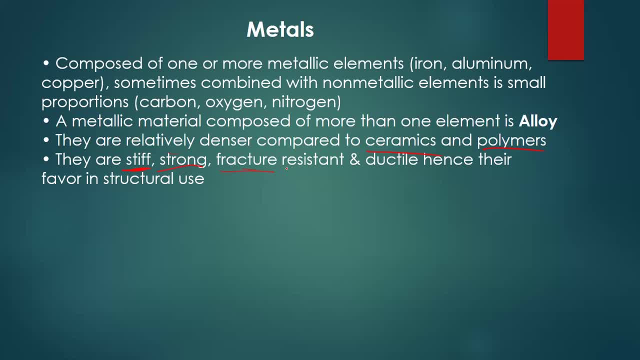 They are strong, They are fracture resistant, They are not fragile. in short, They are adaptor. hence they are adaptor, meaning they can be drawn into wires. They are also malleable, and then malleable, meaning they can be drawn into sheets. 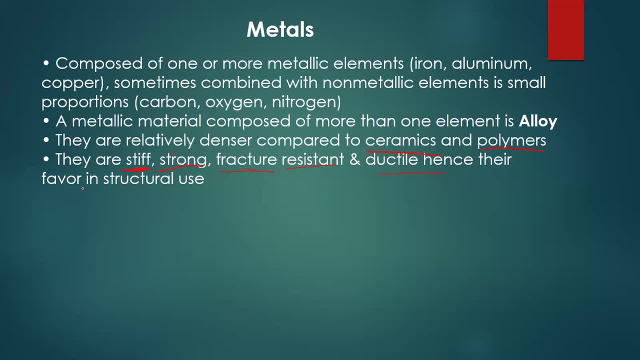 Yeah, so there are a lot of properties of materials, Some of them, I didn't list them here. Then they have non-localized electrons- I think this was discussed in chemistry- which we can also try to research about a bit, because there's a part which we require you to know this. 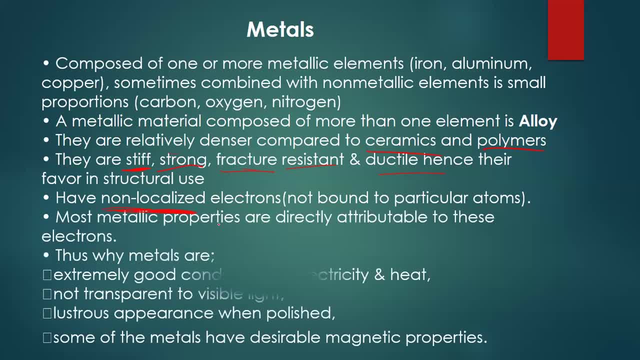 Yeah, so coming to that, Yeah, so most metallic properties are directly attributable to these electrons. yeah, So we know to say they have non-localized electrons. yeah, So most of the properties of metals are attributed to this same property, which is the non-localization of electrons. 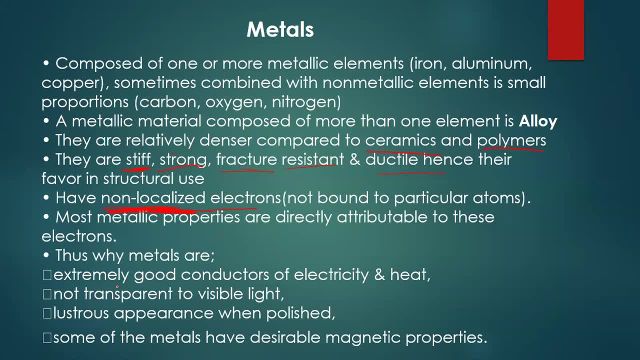 Thus we say the metals are extremely good conductors of electricity and heat. yeah, So we know that electron, rather I mean metals, are good conductors of both electricity and heat and heat. yeah, and then they are not transparent to visible light. yeah, this is obvious, most of the metals. 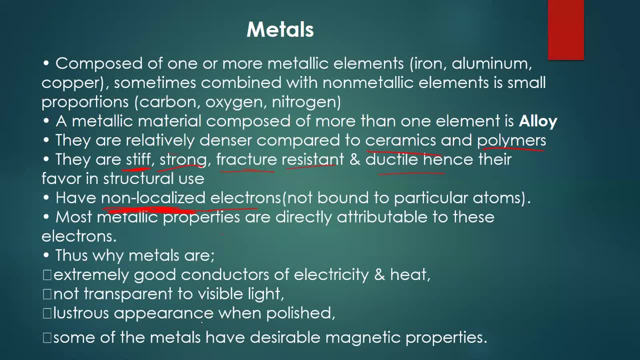 are not transparent. let me just say they are not, yeah, and then we know that they are lustrous. they have a lustrous appearance when polished, meaning they are shiny. then some of the metals have desirable magnetic properties like ion. yeah, we have metals, a lot of metals we have. 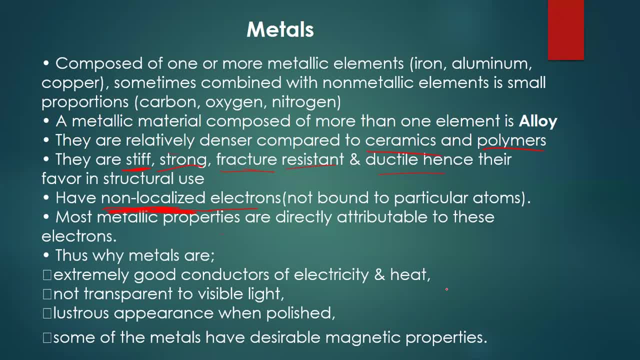 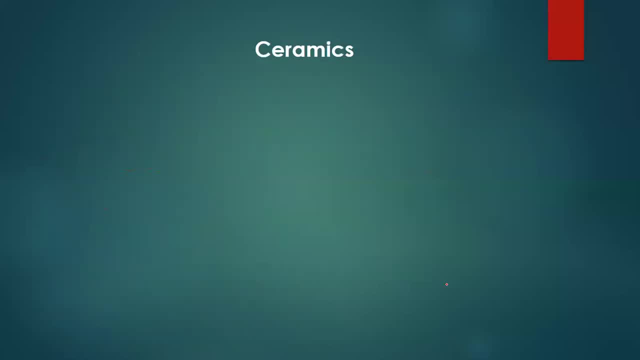 ion. i think there's also another metal which has magnetic properties, yeah, but the one which is common is iron. okay, let's look at ceramics. okay, so ceramics, ceramics- can be metallic or non-metallic. yeah, and for metals, i didn't put any pictures of examples there, because we all 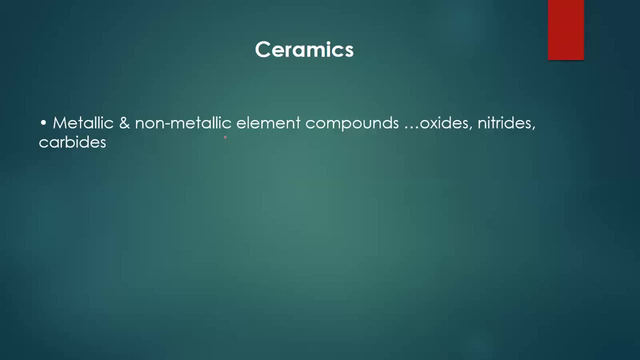 know what metals are, but for ceramics i'm going to put some. i'm going to beam some of the examples here. i think i put some of the examples in the slide. so, metallic and non-metallic elements, element compounds: yeah, so these are oxides, nitrites and carbides. 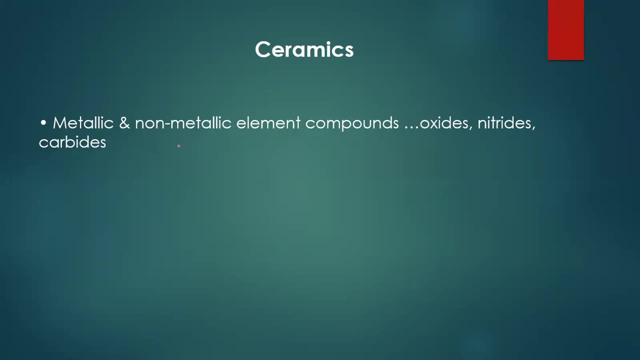 yeah, so ceramics are basically. i mean, ceramics can either be metallic or non-metallic, and they are basically oxides, nitrites and carbides of metals. in short, okay, so so we also have traditional ceramics. so traditional ceramics are, i mean, the examples are clay- we all know what clay is, i'm sure- and then also have cement and glass. so glass, glass, anything. 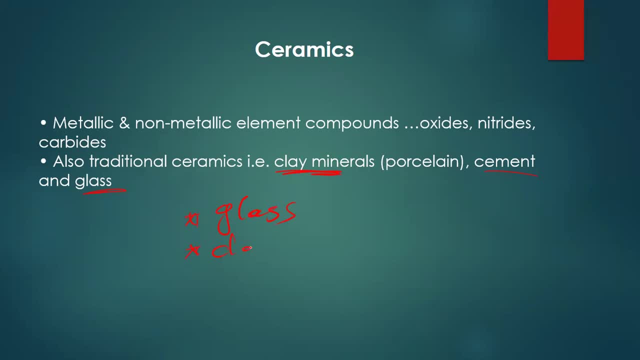 that is made of glass, anything that is made of clay, anything that is made of, uh, cement is a ceramic. yeah, as long as it's pure glass, pure clay and it's pure cement, then it's a ceramic. yeah, so most of these ceramics are brittle. i'm sure there's a. there's a point which i put up, which is in the: 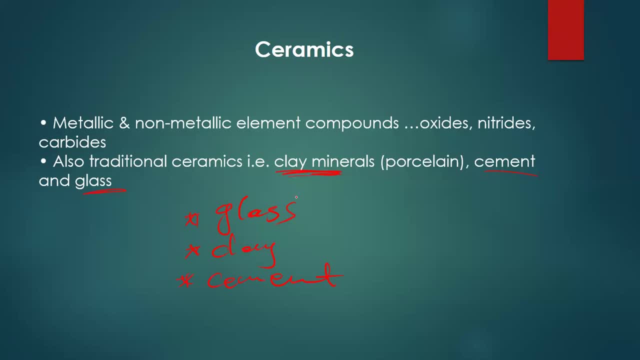 slide. so most of these are brittle. when you, when they fall down on the hard ground, they easily break. yeah, they are brittle and they are hard. they are very hard. some of them are even harder than me those- but they can easily break. okay, so they are strong we have. these are some of their properties. 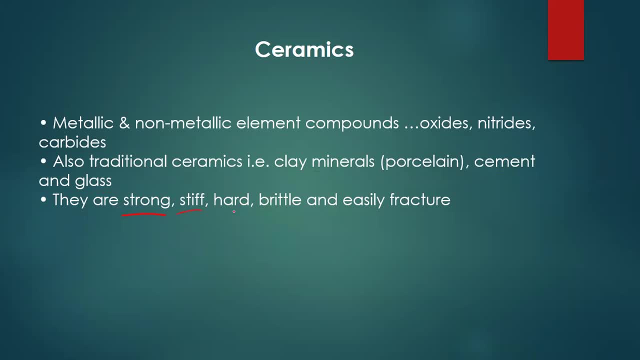 so ceramics are strong, stiff, they are hard, brittle and easily easily fracture. yeah so they are brittle, they easily fracture, they are hard and they are stiff, and most of them are stronger than even metals. yeah, so the insulative um properties of ceramics is quite high. yeah, so some, some of the ceramics are even used at the 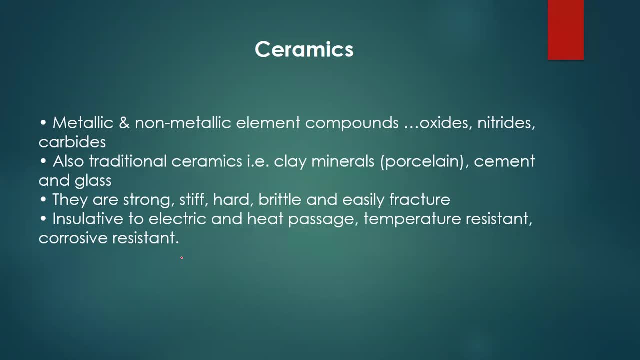 pores. i'm sure you've seen those round things round brown things which are, um, which are connected to power, i mean to power cables. yeah, there is that cable. if you have a pop, if you have a pole which is, let's say, we have a pole here, then it has some cables which have been connected, going like this: 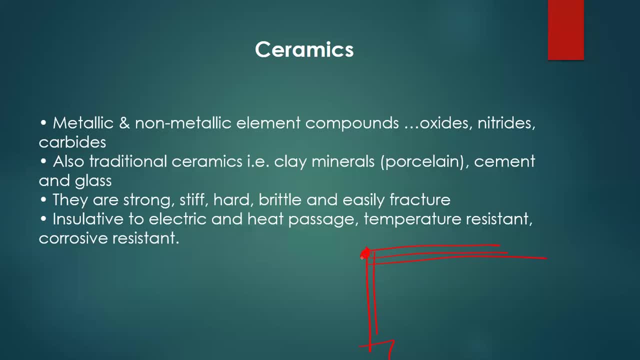 if you have observed it, there's this: there's always this cable which is connected to the pole and then it's also connected to the ground, but before it reaches the ground there's one component: brown brown. sometimes they are white, yeah, sometimes they are whitish. yeah, milkish color, i don't know that color. some of them. 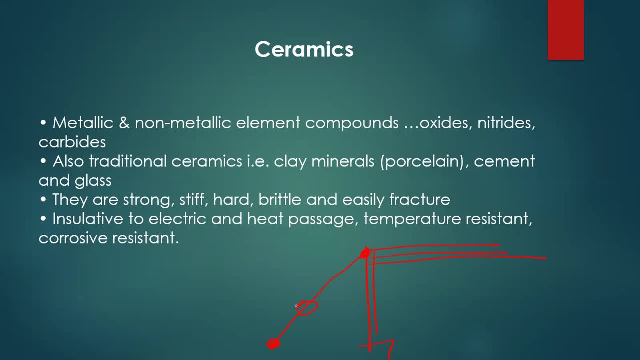 they are brownish. yeah, so there's that component which connects this cable. there's that component. it looks like this- let me just try to sketch it: so you have a cable coming from this side and then another cable this side, then you have something here in between. so this thing is the one that we call. i mean, this thing is: 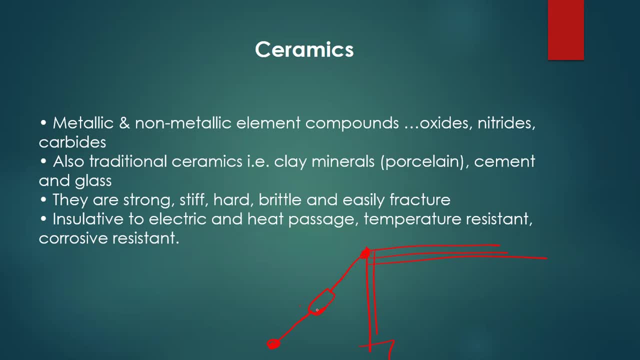 made out of a ceramic. and the reason as to why they use uh ceramics to make this uh thing? because they know to say: ceramics do not conduct electricity. they are very poor conductors of electricity. hence, if they connect it like this, even if a person touches this part of the 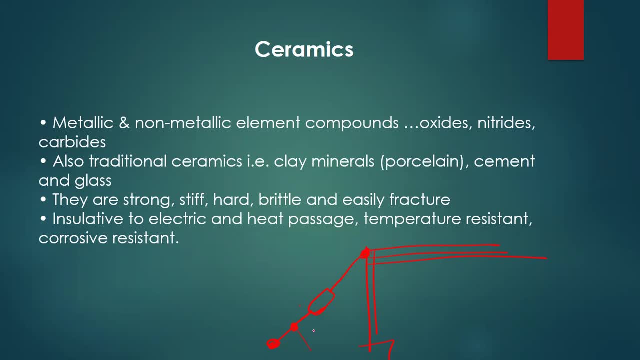 cable, they will not get electrocuted. yeah, they will not get electrocuted, but if you touch this side, maybe this side, this, this part, can even be connected to one of the cables, this side. hence, maybe, if you touch it, you might even get, uh, shocked, but when? 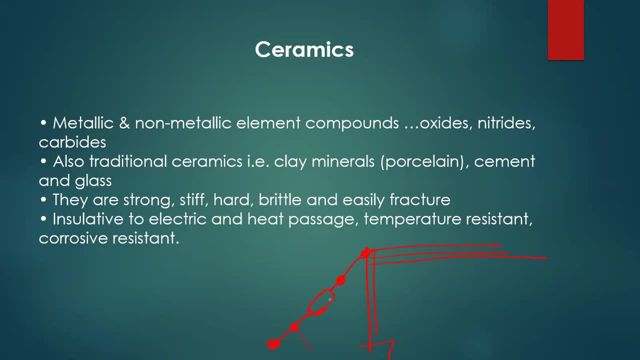 you touch this side, you can't be shocked, because there's a ceramic in between here which is a very bad conduct of electricity. yeah, and not only electricity. they are also very poor conductors. they are very bad conductors, rather, of um heat, yeah, temperature. they are temperature resistant and corrosive resistant. they don't easily corrode. 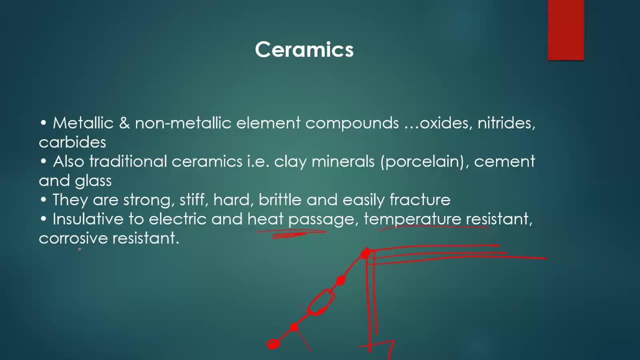 yeah. so i'm sure you guys have seen these things before. you didn't just know what i mean, maybe the time i introduced them. okay, so some of them may even be transparent, like glass. we know glass is transparent, then translucent, then some of them may be open. 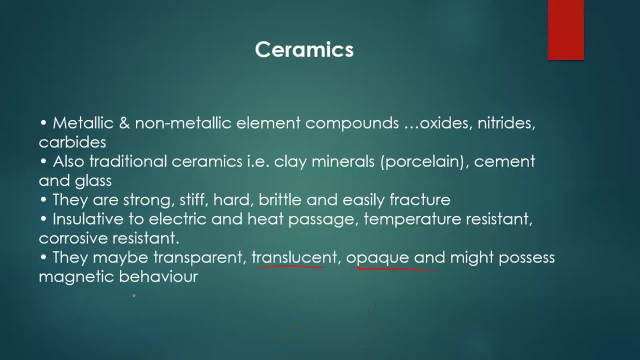 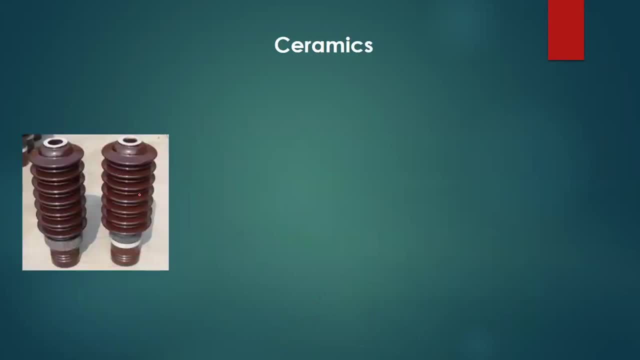 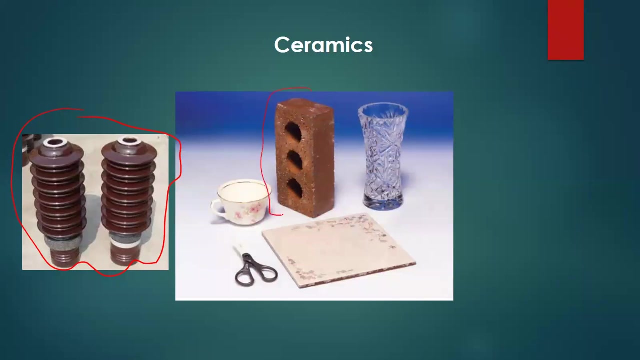 then they might, might, possess magnetic, uh behaviors. yeah, so this is. these are some of the examples of ceramics. i'm sure you guys have seen this on the pause, uh, on zesco gen sets. all these things are made of ceramics. then there's also these things, we know these things. remember what i said: cement is also one of the ceramics we have. 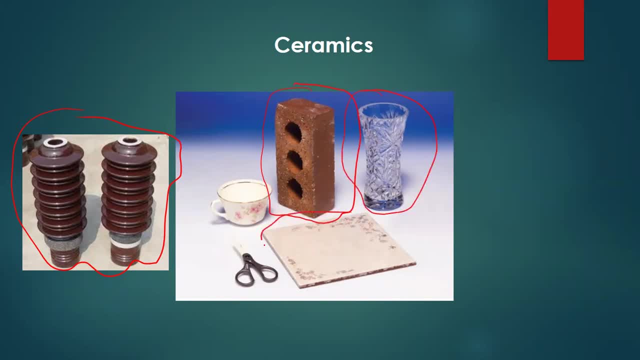 glass, which is also a ceramic. We have towels. Towels are also ceramics. Then there's also this here, which is made of a ceramic. We also have this breakable. I'm sure if you research properly, you'll discover that this breakable is made out of clay. 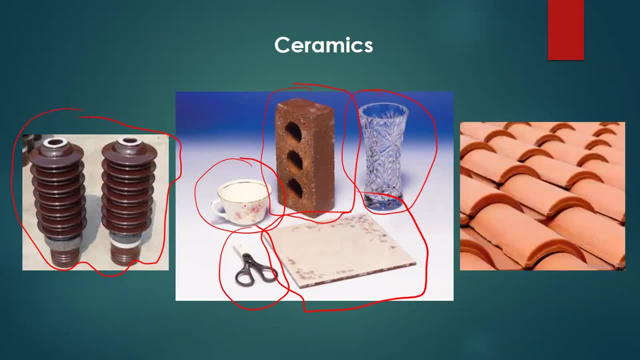 So it's also a ceramic. OK, we also have these types of roofing sheets. They are also made out of ceramics, So I'm sure you've seen these somewhere before. They are easily breakable. When you drop a glass down, it easily breaks. 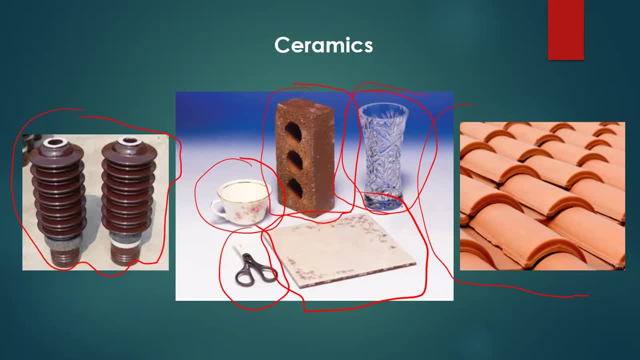 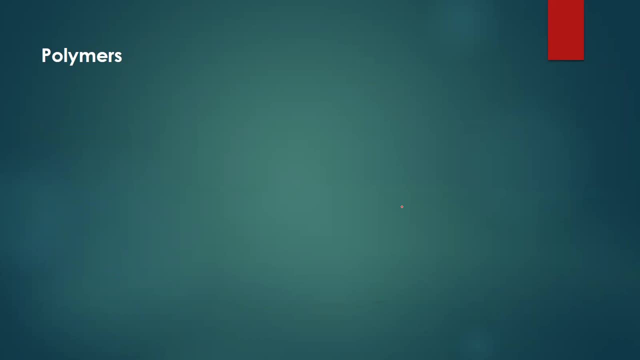 So those are some of the properties of ceramics. OK, let's move on to the next one. We have polymers. So polymers are exactly the same things that you learned in chemistry. So most of them are organic compounds chemically based on carbon. 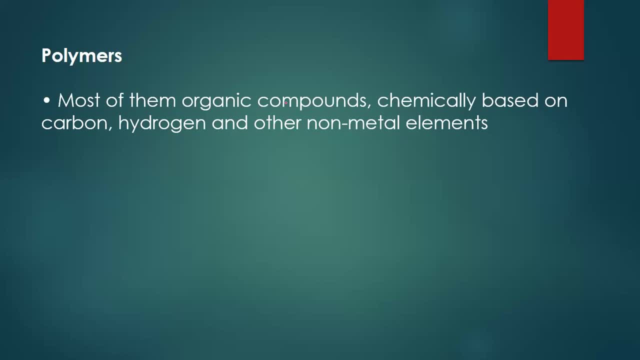 Hydrogen and other non-metallic elements. Yeah, so polymers are basically. I mean, they are basically organic compounds which are a combination of carbon and hydrogen and also other non-metallic elements, And then they have large molecular structures. I'm sure you learned about this. 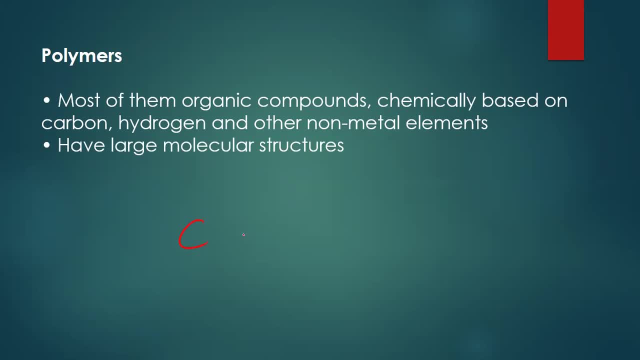 They have large molecular structures, So their chemical compounds are mostly in this format. You have a lot of carbons in them, So you have something like this. You can even have maybe an oxygen element there. OK, so polymers. you discussed this in chemistry and I'm sure you know them. 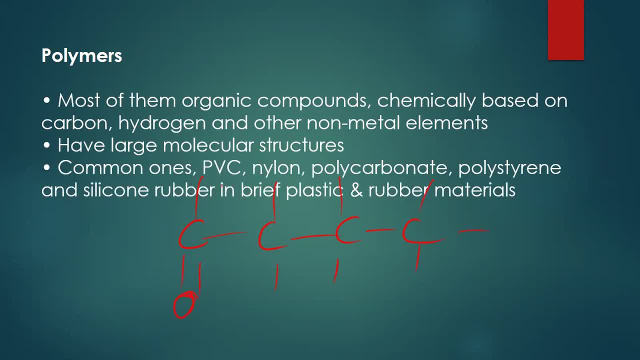 So let's just look at some of their properties. So some of the examples: we have PVC, polyvinyl chloride, We have nylon, We have polycarbonate, We have polystyrene And silicone. I mean silicone, rubber, in brief, plastic and rubber materials. 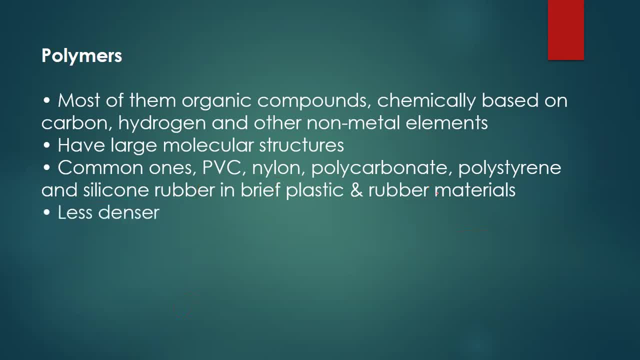 So most of the rubber materials are polymers. Yeah, so these are some of the properties. We know that polymers are less denser. Then they are not stiff. They are not even strong. Yeah, I'm sure you are taught that in chemistry. 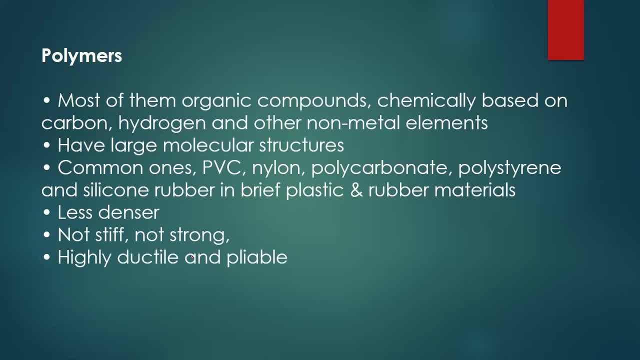 Then they are highly ductile and pliable. And then, apart from that, the polymers chemical in it, meaning they are not reactive- Most of them are not reactive to chemicals- And then they are corrosion and reactive. Yeah, All right. so 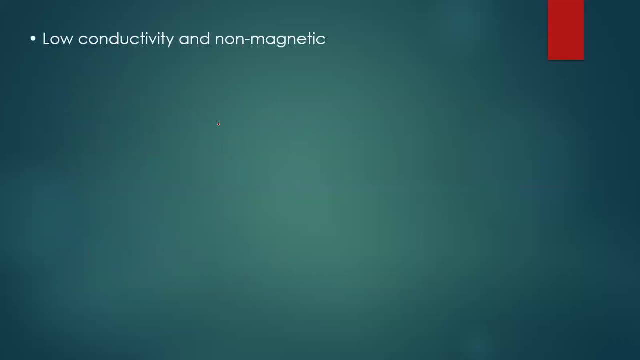 They also have low conductivity And non-magnetic. Most of them are non-magnetic. Let me just say, oh, because I've never seen a polymer that is magnetic. Yeah, I think I saw one. OK, I'll try to research on it. 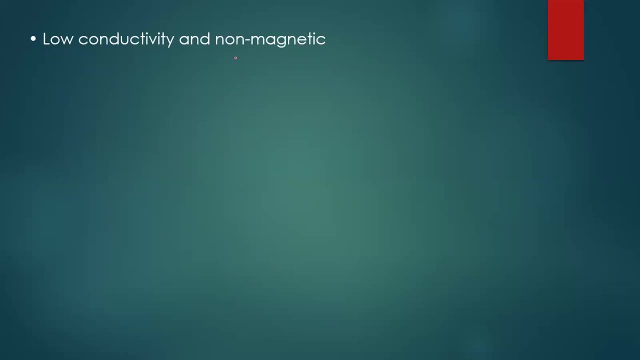 Anyway, yeah so most of them are non-magnetic And then they have low conductivity. Yeah So, and then they have limited use. I mean, They are used, They are normally not. They are usually not used in making some of the things. 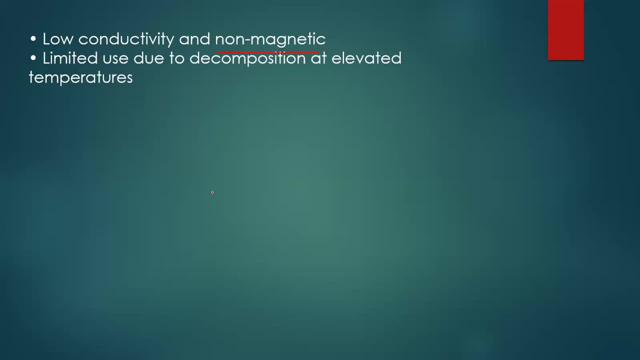 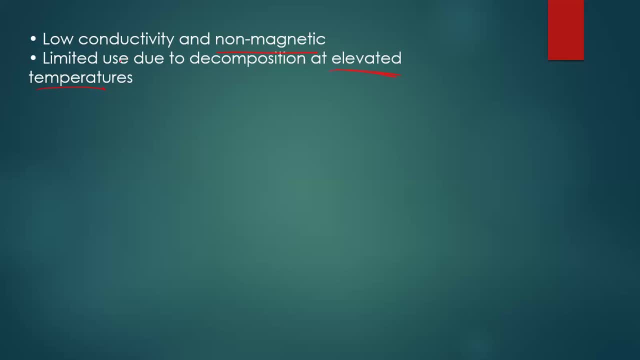 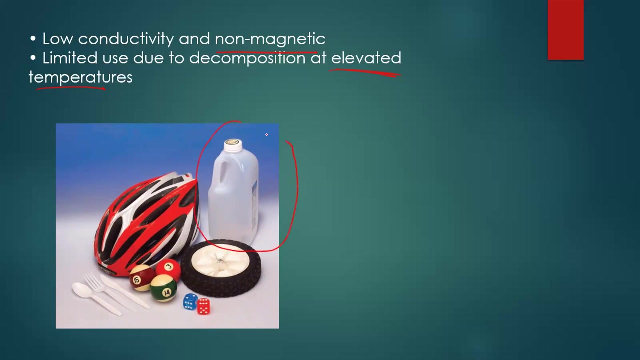 So they are not usually used in things or in making things that have, or that undergo, very high temperatures. Yeah, So these are some of the examples of polymers or things that are made of polymers. We have this plastic bottle that you are seeing here. 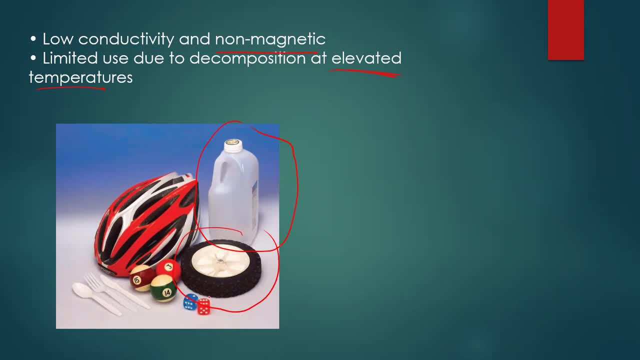 It's also this rubber tie that you are seeing there, And then, apart from that, we also have these dices, And then there are also these pool table balls. Then we have these plastic spoons there, a fork and a knife. There's also this. I think this is something that they use, that people use when they are cycling, if I'm not mistaken. 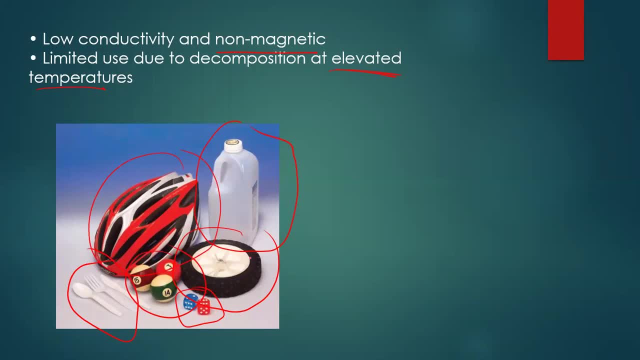 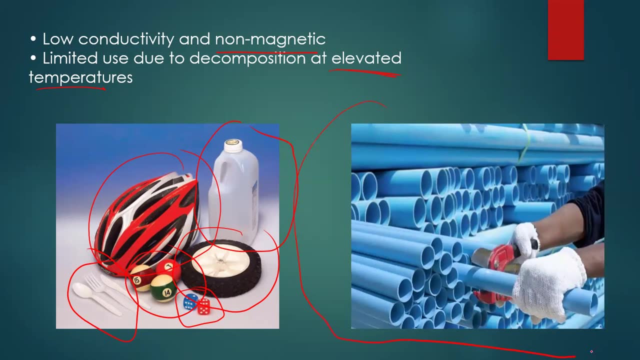 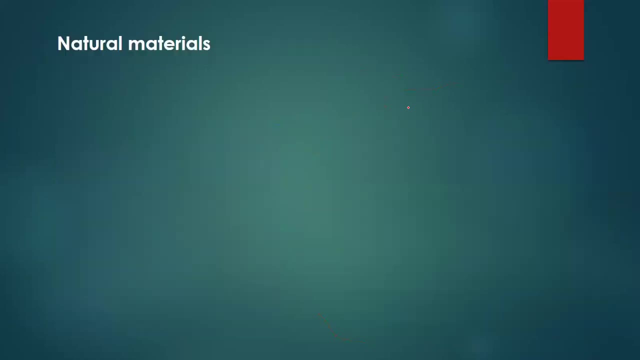 Yeah, So as long as it's made of something that is rubber, it's a polymer, All right. We also have plastic pipes, So plastic pipes are also polymers. Yeah, They're also made of polymers, All right. So I think, oh, I don't. that was the end of the lecture. 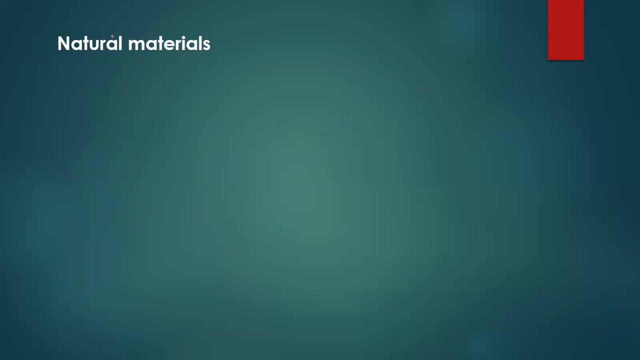 I still have some more slides, All right. So we also have what are known as natural materials. So natural materials like gravel, we have the rock, Then we have bitumen, wood lathes And then we also have plastic pipes. 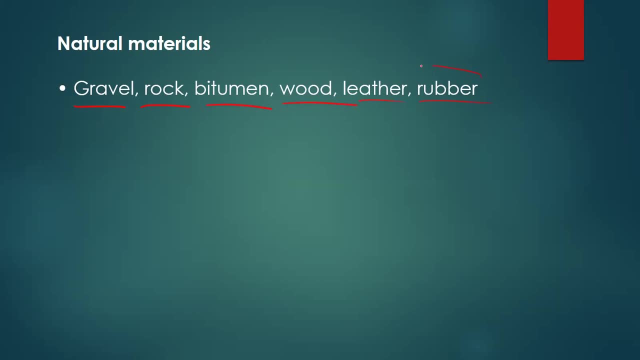 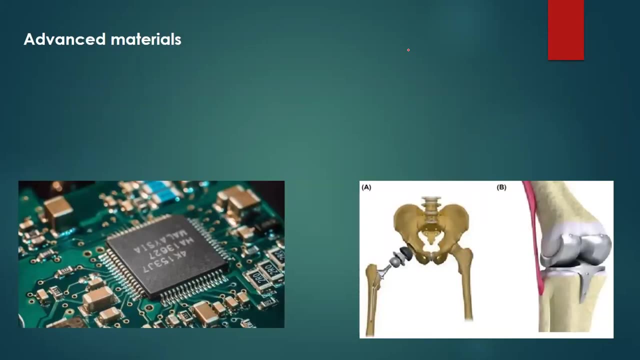 So plastic pipes are also polymers, And then there's also rubber- though rubber falls under polymers as well- And then we have advanced materials. I talked about advanced materials, Yeah, So all these, all these components that you are seeing here, all these components that are made of- let me just say, this component you are seeing here, it's made of what is known as an advanced material. 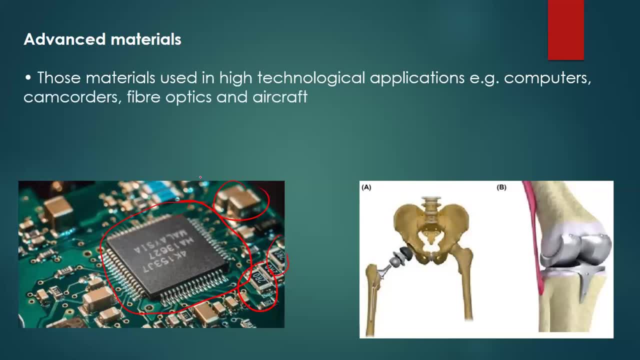 Yeah, So those materials used in high technological applications, eg computers, camcorders, fiber optics and aircraft? Yeah, So this is not I mean in material science. yes, we'll have a lot of notes for you to write, but there are also calculations that are going to be doing. 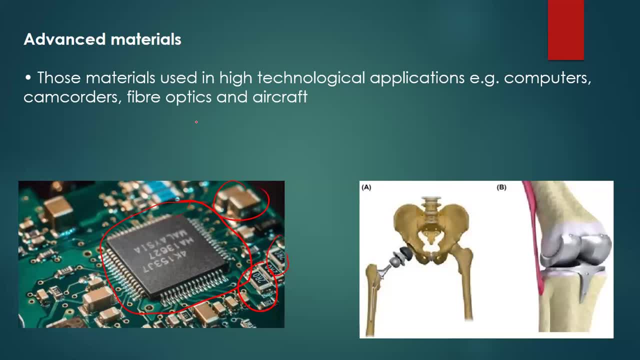 For now, I think we'll be having notes for, I think, for a continuous, maybe three or four lessons, But after that we'll have a lot of calculations Which you need also to know. All right, So we also have this. 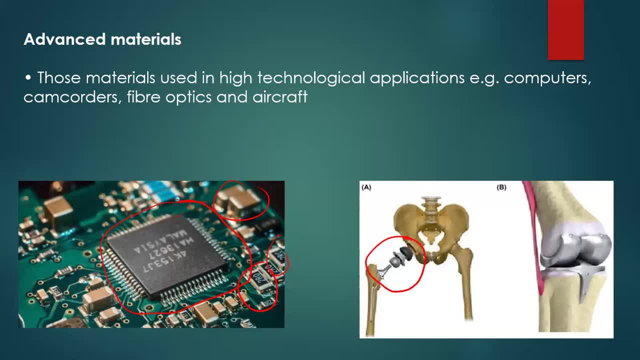 You can see, these are biomaterials. Some of these can be called biomaterials Because they have been made out of these same advanced materials. Yeah, So some of the examples are semiconductors. Then, apart from that, we also have biomaterials. like I said, 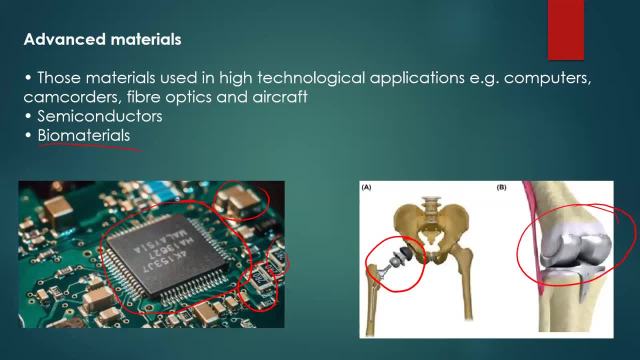 Yeah, These are artificial. I don't know what you call this part of the bone. Then we have smart materials as well. I talked about this at the beginning. All right, So thank you very much for attending tonight's lesson. These are notes. 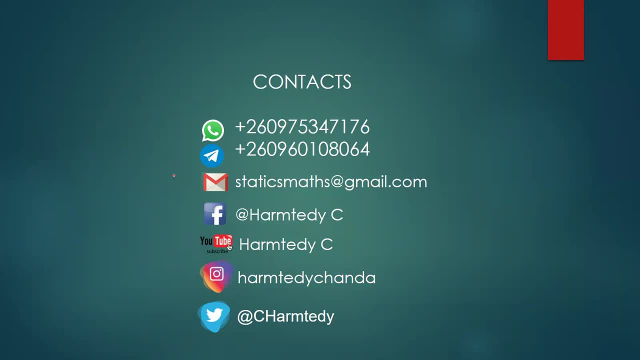 That's why I didn't allow questions. You can easily just even research, Yeah, So when you start doing calculations, where you need to understand, I'll be making sure that I explain. So I just went through these slides quickly, Because these are just notes. 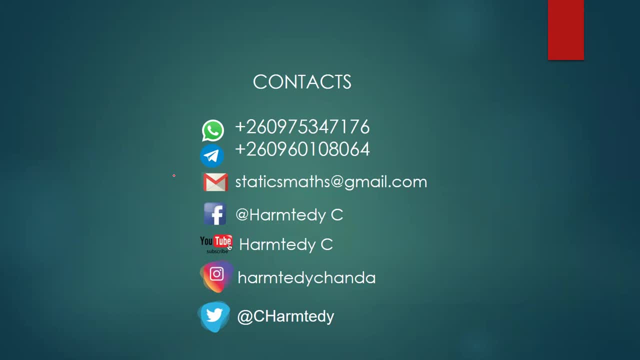 Moreover, I'm going to send the slides to you, Yeah, And you go through them. So just make sure that you know more, especially the properties. So I know most of the lecturers at MU they ask They don't leave those questions about properties of these materials.